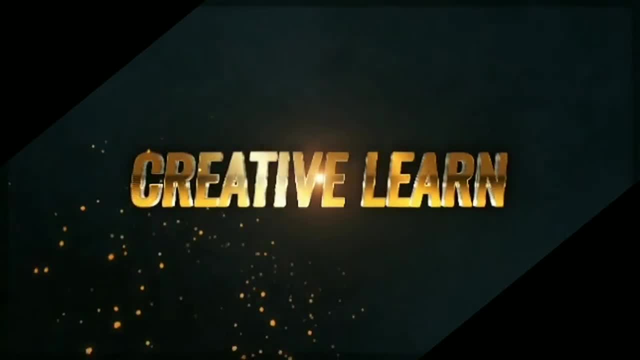 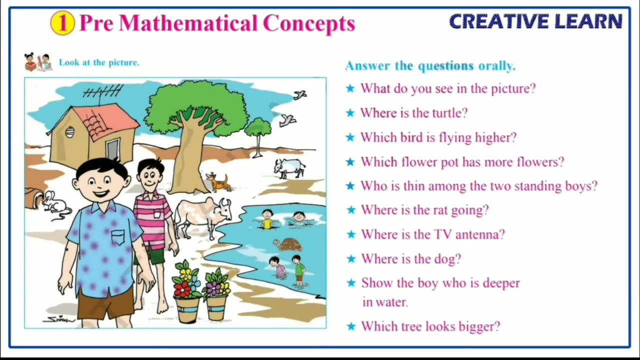 Hello everyone, welcome to CreativeLearn channel. Today, in this video, we are going to discuss about three mathematical concepts. Okay, here, one picture given. Let's have a little conversation on this picture. What can you see here? House trees, birds. two boys are standing rat. 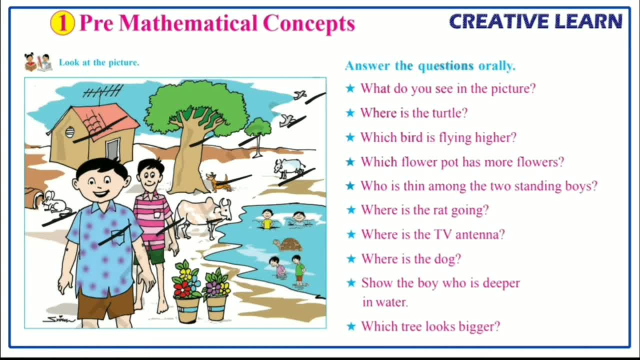 two cows also there dog, two flower pots with beautiful flowers, some boys are getting fun in water and one turtle. Okay, this is about picture. Here, some questions given related to picture, So let's try to answer these questions. Okay, what is the first question given? 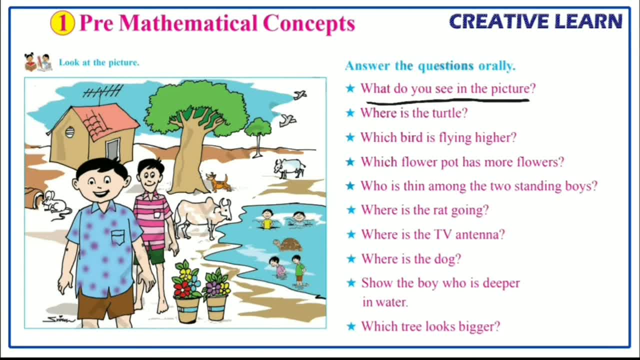 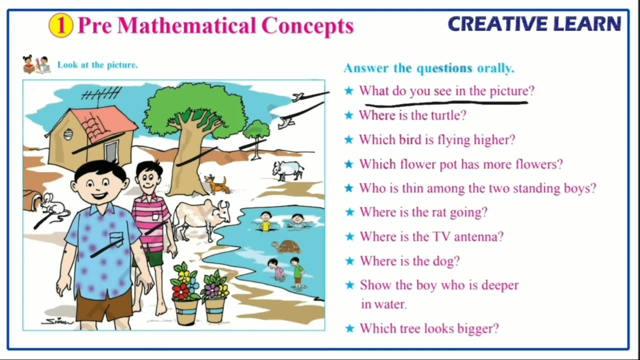 First one: what do you see in the picture? Just now only we said: what do you see in the picture? House tree birds, two boys, one rat, one cow here, another one also there, and two flower pots. and some boys are getting fun in water. Here one dog. 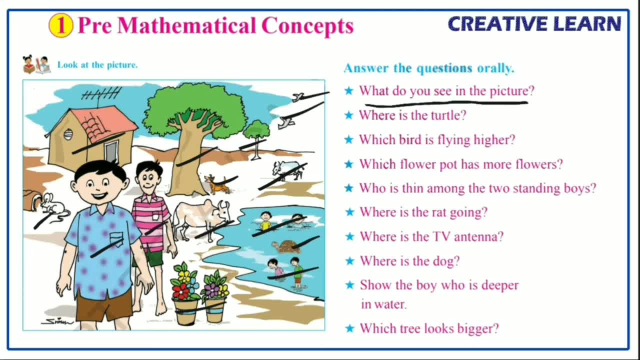 and here one little turtle also there. So this is about the first question. Now what about the second question, Turtle. So in the whole picture, where is the turtle Here? Here is the turtle. Turtle is in the. Where is the turtle? Turtle is in the water. Now, which bird is flying higher? What is the third question? Which bird is flying higher? 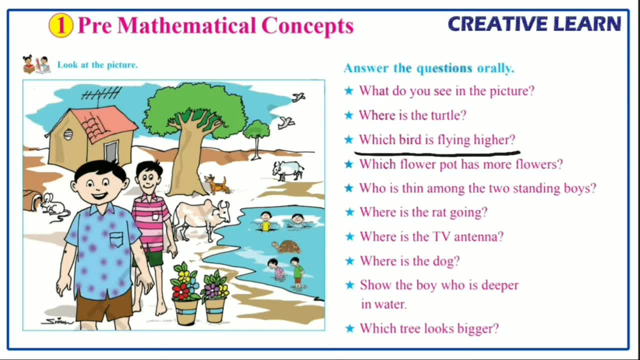 So, in the picture, two birds are flying From these two. which one is flying higher? This bird is flying higher compared to this bird. Now, what is the fourth question? Which flower pot has more flowers? so here in the picture, two flower pots are given from these two. which one has? 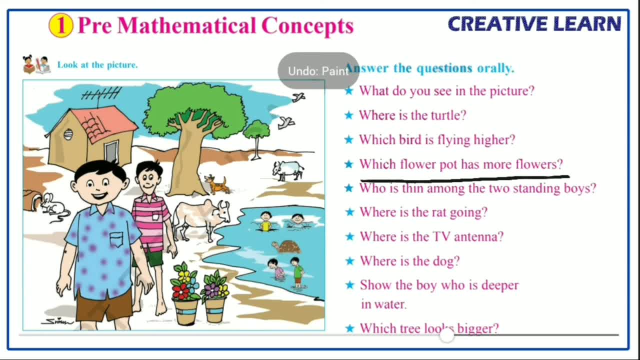 the more flowers shall we count? from the first flower pot we have one, two, three, three flowers are there now? from the first flower pot and from the second flower pot? we have one, two, only two flowers now. tell me which flower pot has more flowers. first flower pot has more flowers. which flower pot has more? 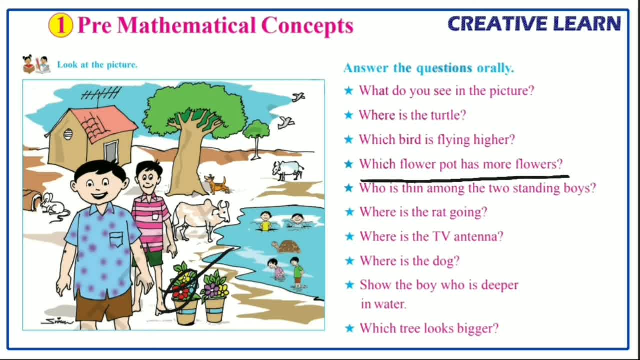 flowers. first. flower pot has more flowers. now let's go to next question: who is thin among the two standing bones? so in the picture two boys are standing here. from these two standing boys, who is seem to be thin? so this boy is looking thin compared to this boy. Okay, Next. 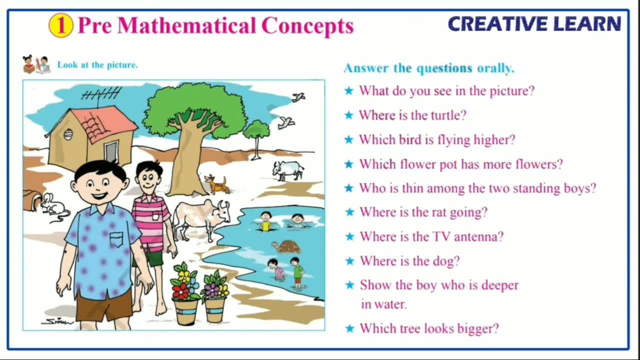 question here. next question. Okay, next question here. next question: Where is the rat going? Okay, in the picture, where is the rat? Haa, here is. So where is rat going? Rat is getting into burr over. Where is the rat going? 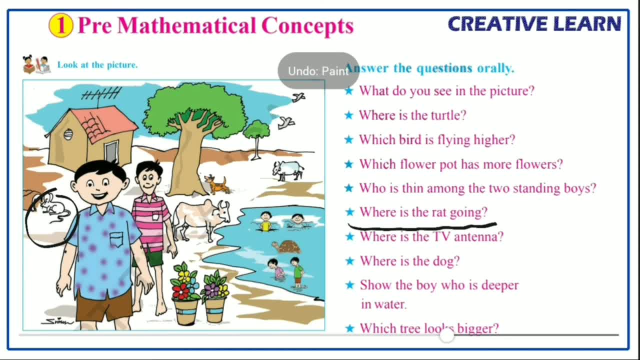 Rat is getting into burr over Now. next question: Where is the TV antenna? Where is the TV antenna? in the picture Here is TV antenna is on the roof of the house. Where is the TV antenna? TV antenna is on the roof of the house.